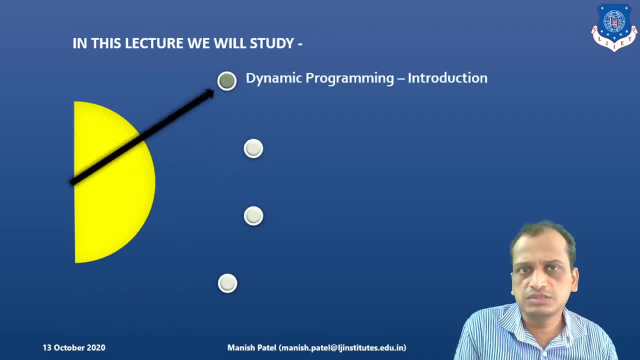 of all, we will learn what the dynamic program is. what are the concepts related to dynamic program? Then we will look into the terms that are related to dynamic programming. We will also look into the characteristics of dynamic programming And finally, what are. 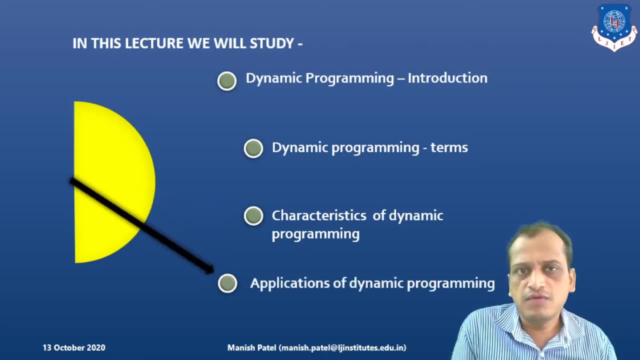 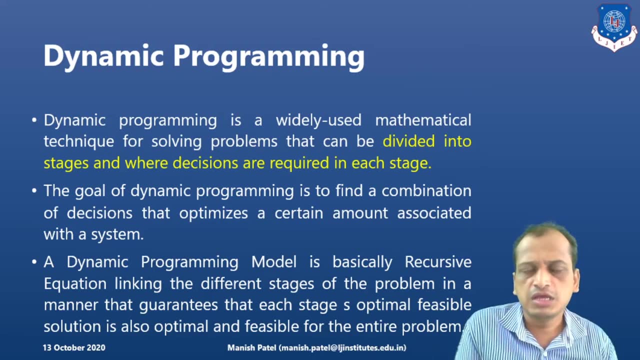 the applications of dynamic programming. Where do we use or where do we employ dynamic programming yet? So let us start with the dynamic programming. What dynamic programming is? What do we mean by dynamic programming Here? in linear programming problems, the problems were of linear type, right The functions. 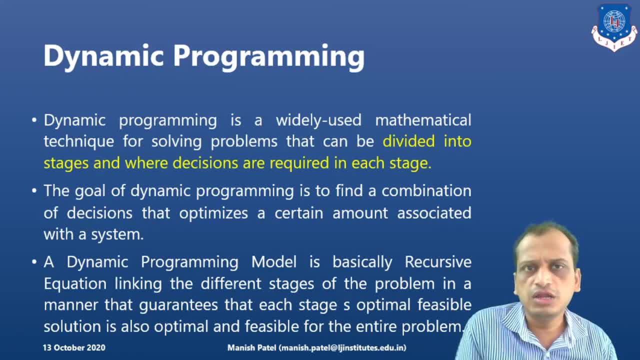 which were involved: objective functions, constraints. they were of linear type. Now, specifically in dynamic programming, the problem is divided into different decision stages. Now, at each stages, the decisions are to be made And we have to find out the optimal. 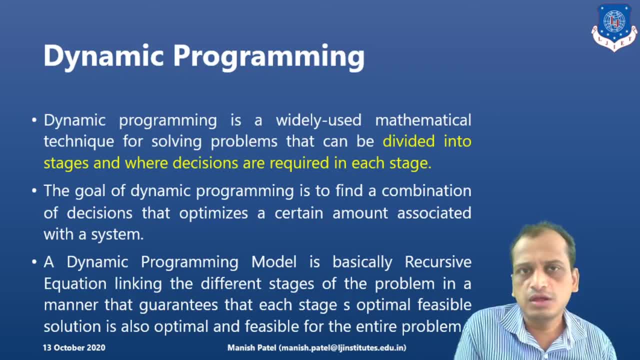 decision making for the entire problem right. What we try to do is at each stage we will find out the optimal solution for each decision making, And then the constitution. the whole problem is literally divided into different stages. For each optimal stage, we will try. 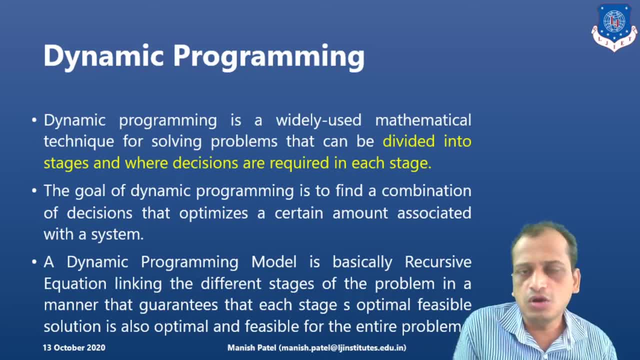 to find out, for the entire problem as well, the optimal solution right- And it is definitely. it is basically the goal for the dynamic programming- is to find out the optimal solution out of this decision making problem right By dividing the problem into two. So we will try to find. 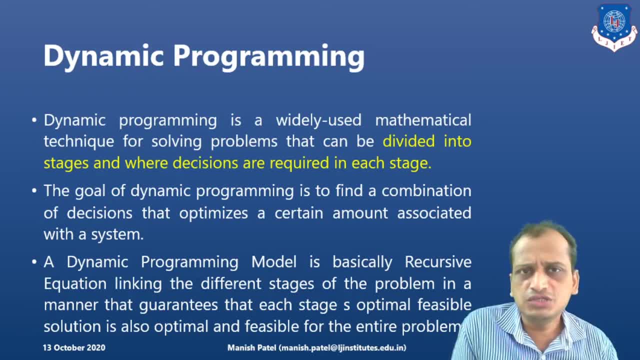 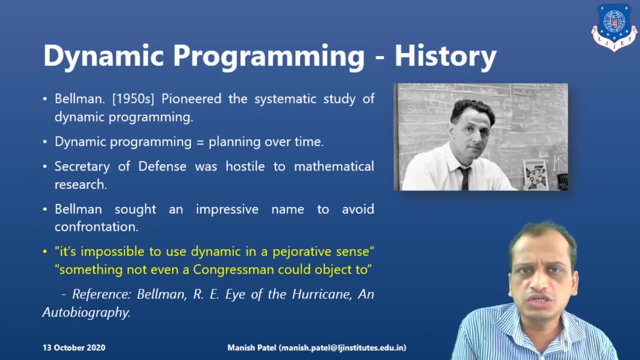 out the optimal solution out of this decision making problem by dividing the problem into different stages. The nature is of recursive equations. What do you mean by that? That each stage, the feasible optimal solution for each stage, will guarantee that you will get the feasible optimal solution for the entire rate. Now, if you look into the history, 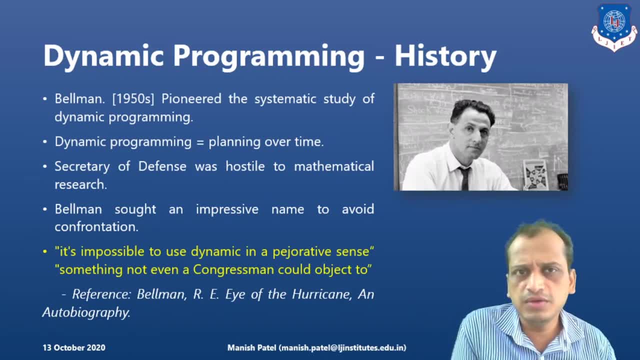 of dynamic programming. it started with Richard Bellman who invented this technique of dynamic programming, But initially he thought of naming it as mathematical research, but it was against the principle of dynamic programming. So he thought of naming it as mathematical thinking of the defense management, but against this mathematical research into this defense. 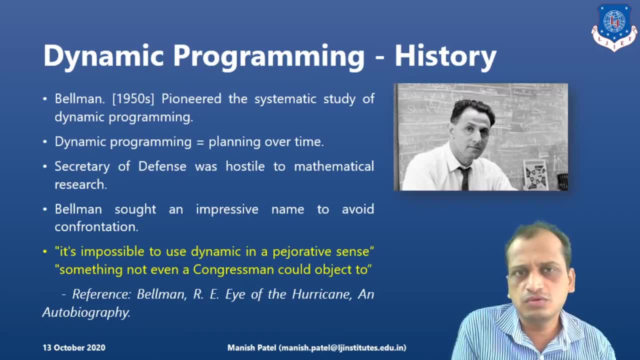 activities. So what he did was he tried to convert this name. he tried to convey the meaning, or you can say the planning over time with a new name of dynamic programming, which would be the less resistance from the defense management at that time. So, according, 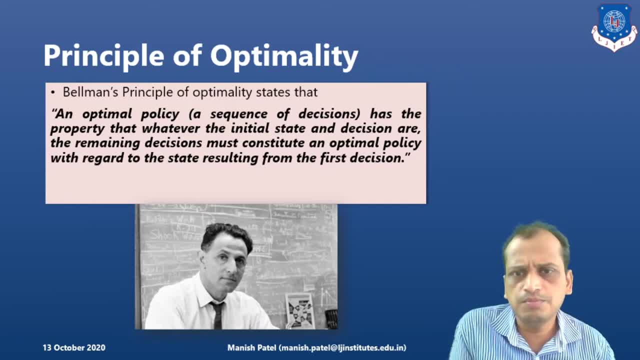 to him, the principle of optimality is an optimal. You can see the sequence of decisions of a problem as the property that, whatever the initial state and decision are, means. whatever you have decided at the initial phase of time, at initial stage, the remaining decision must constitute an optimal policy with regard to. 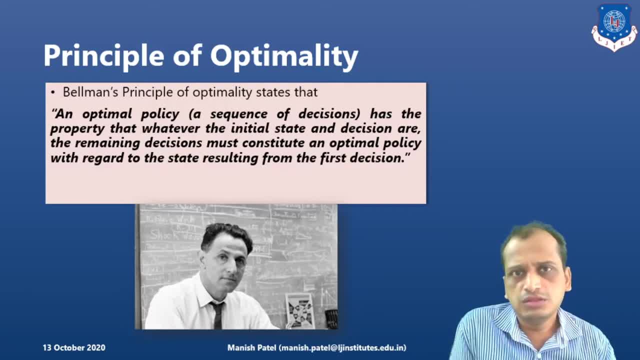 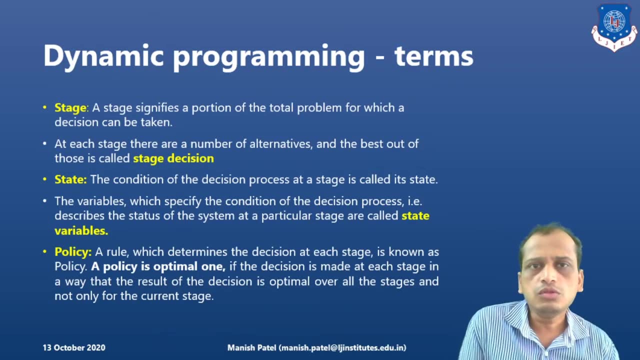 the state resulting from the first decision Means the following decisions that are made, all they are following with the optimal policy which was taken During the first decision. right It also should constitute that optimal policy. So let's look into the different terms that are related to dynamic programming. 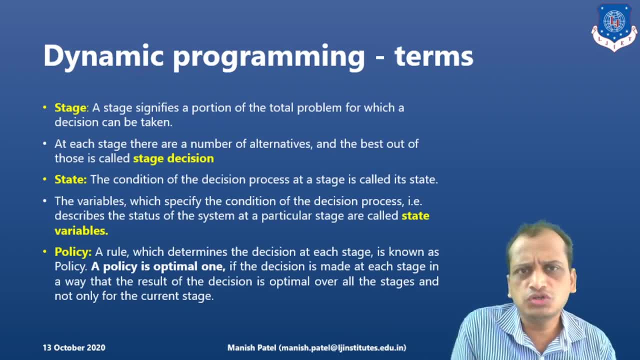 The first of all, it is stage. Stage is nothing but a portion of the whole problem, where the decisions are to be made, And the problem is divided into different stages. right At each stage, different options are there for the decision making right. 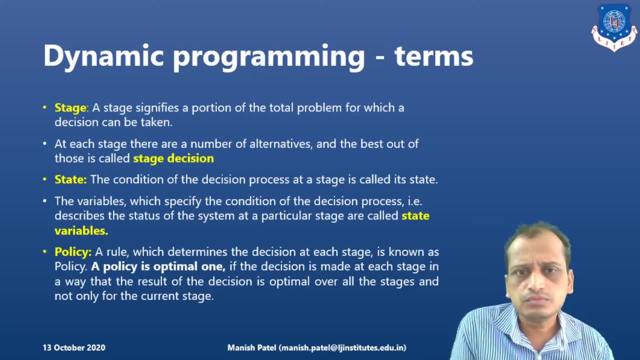 But the best one is called the stage Stage decision. Now, talking about state, the condition of decision making process, the decision process. the condition is called the state and the variable which describes or specify this condition are the state variables. right? 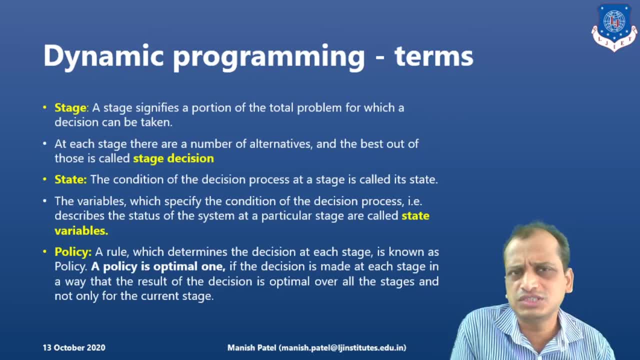 Or you can say: they also describe the status of the system at every stage. That is the state variable. What about policy? These are the rules that define. so you can say: determine the decision at every stage. That is nothing but the policy. 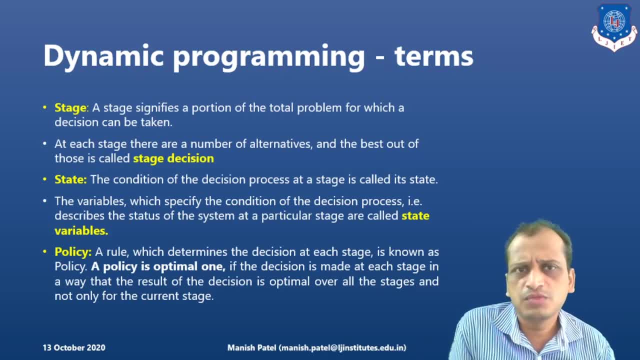 Okay, And optimal policy is the policy which guarantees that you will get the optimal solution, or you can say the optimal decision making, for the entire region of the problem. Also, it is at each stage, it is the optimal as well. right? So these are the terms that are related to dynamic programming. 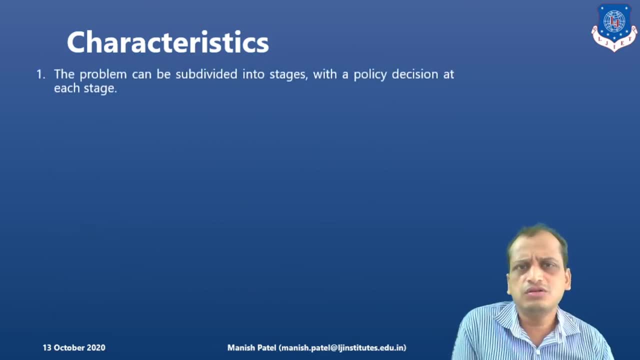 Now, what are the characteristics of dynamic programming? First of all, the first and the foremost one is that the problem is divided into different stages and the decisions are made in the stages. Again, decisions have different types of or different state states, depending upon the 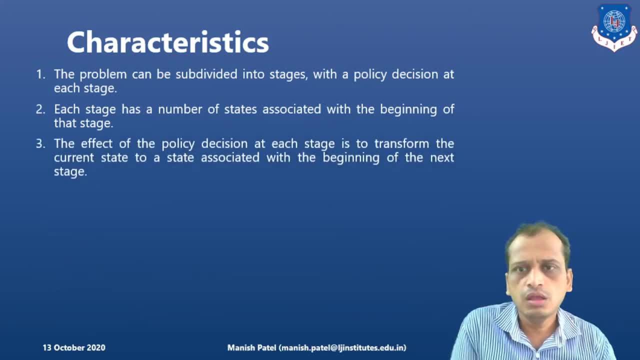 stages And the transformation of state now from the initial state to the intermediate, intermediary or you can say, the final states. different states are there according to the stages of the problem And the focus will be to find the optimal solution Now. even so. 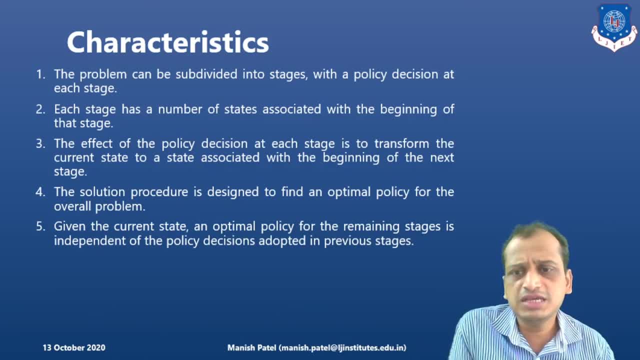 Okay, So the current state, the optimal policy of the remaining states, is independent of the policy decision that are made in the previous stage. Remember this thing. So, whatever the optimal, whatever the optimal policy of the current stage is the remaining, 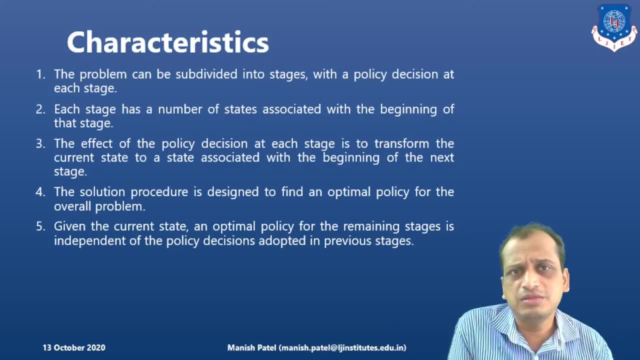 states that is independent of the policy decisions that are made in the previous stage. Then the solution procedure begins by finding the optimal policy for the last stage. What do you mean by that? The problems can start with the last stage. Okay, So the last stage where you have the optimal policy and you go backwards? 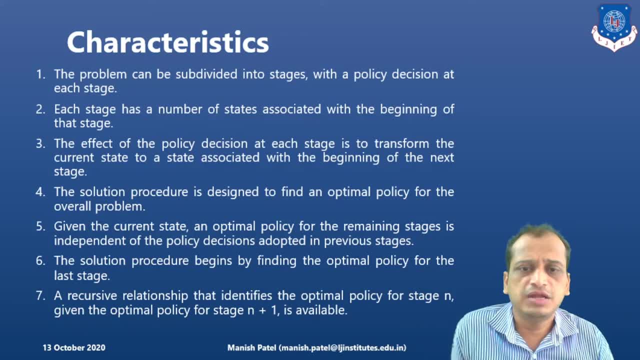 That is the recursive nature of that dynamic programming. That is the recursive relationship. It means that let's say, for example, optimal policy for the stage n plus one is there. So the optimal policy for the stage n that will be identified based on the optimal policy. 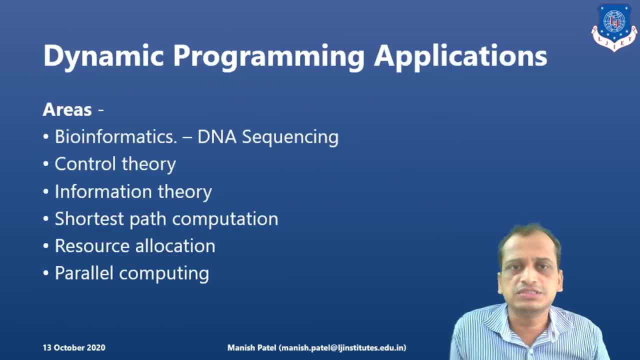 of n plus one Means recursive Right. So what are the applications? Where do you use dynamic programming, Specifically In DNA sequencing? If you talk about in biology DNA sequencing, then control theory, control engineering, information theory, computer science, parallel computing, resource allocations you have. 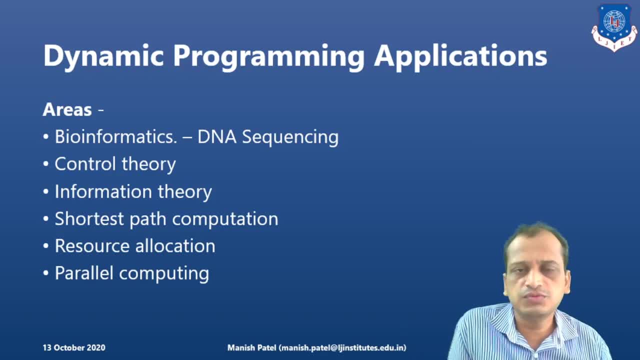 specifically in supply chain management, in defense as well. Then you have shortest path computations, let's say, for example, from A to B. if you want to travel- And they want to have this- Have the shortest path available. The best example is Google Maps, where you want to try to go to specific destinations. 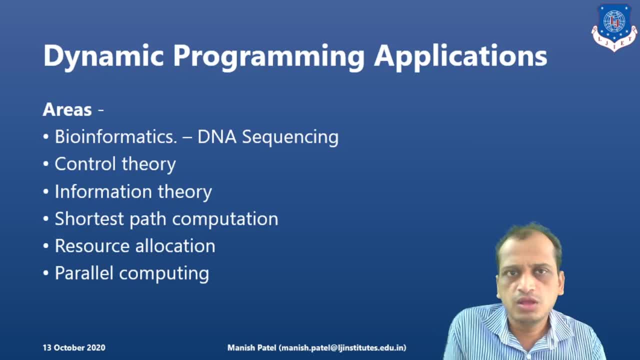 and then, if you want to find the shortest path, the Google Maps employs this dynamic programming algorithms to find the shortest path available This way. these are some of the many applications of dynamic programming. You can employ this algorithm, which is divided into different stages and each and every stage.